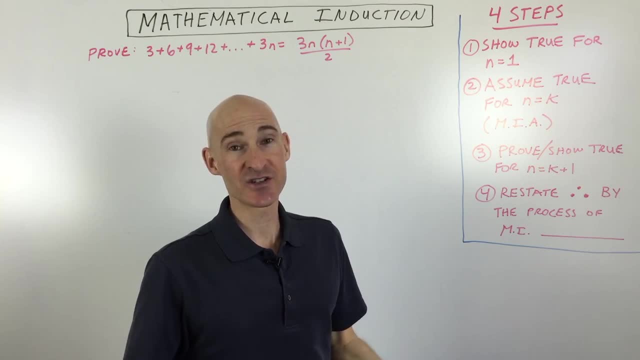 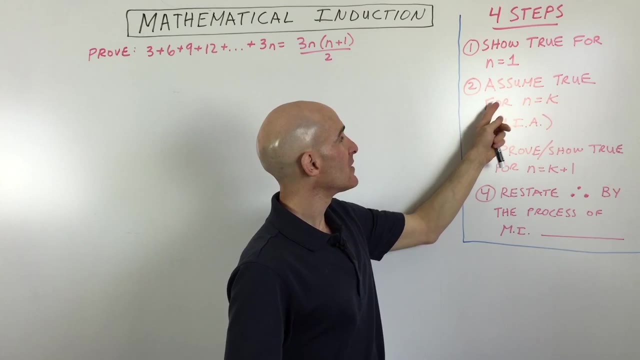 doesn't work for the first term, then you know it's just not true, so there's no sense in proceeding from there. Okay, so then you go to the step number two and you make this assumption. You say: let's assume that this pattern, okay, this theorem, this formula is true for n equals k. 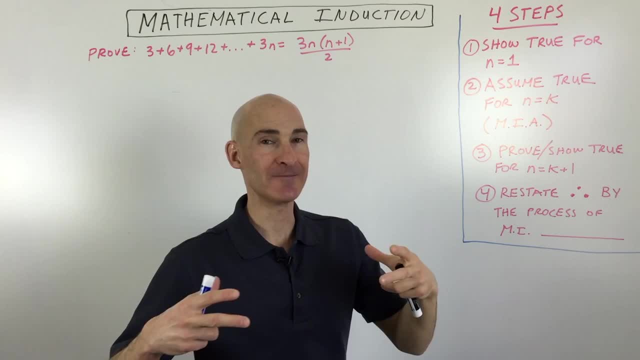 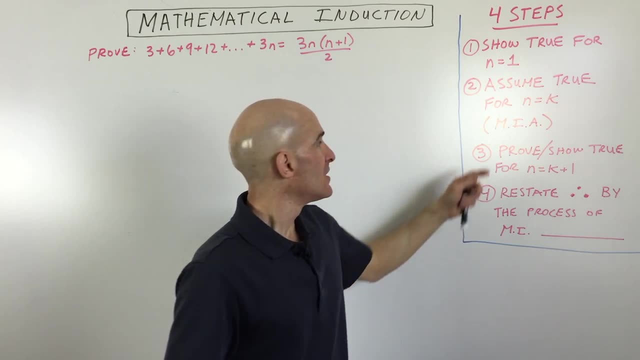 Now, n is the number of terms and k represents, like you know, like a set number of terms, like five terms, ten terms, like a fixed number of terms, And this is called the mathematical induction assumption. Just I abbreviated it here: MIA: mathematical induction assumption. So you, 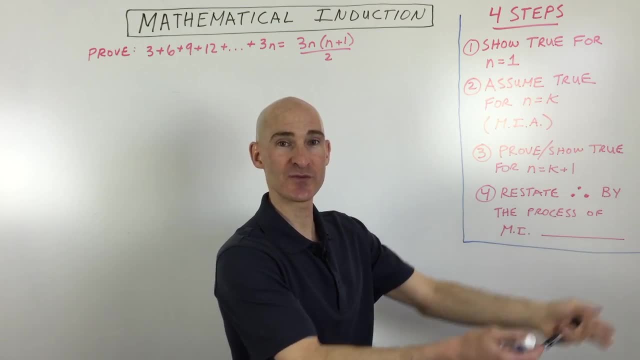 make an assumption that it's true. you know and you can show that it's true for two terms, three terms, four terms, five terms, six terms, seven terms, eight terms, nine terms, ten terms, nine terms. But when we get to step number three, what we're trying to do is we're trying to prove, or? 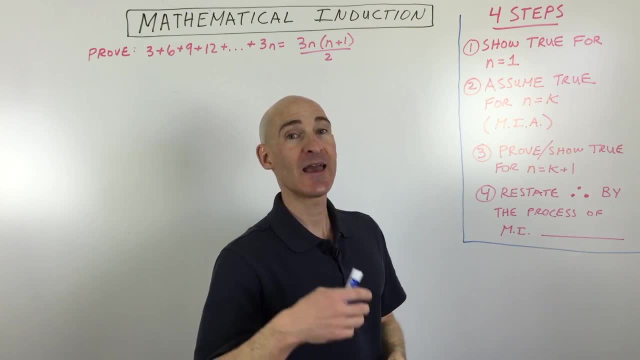 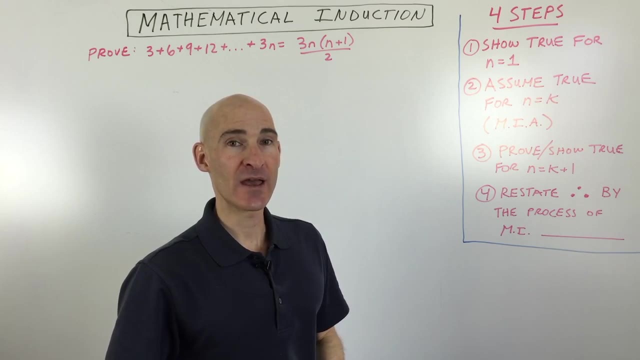 show that it's true, for n equals k plus one. So that means like one term beyond that fixed number of terms, k. okay, Because if it works for one term beyond that, it'll work for one term beyond that, and beyond that add infinitum, right forever. So then the last step, once you've proven this. 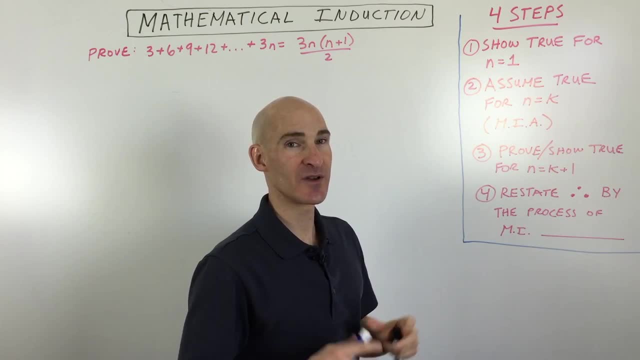 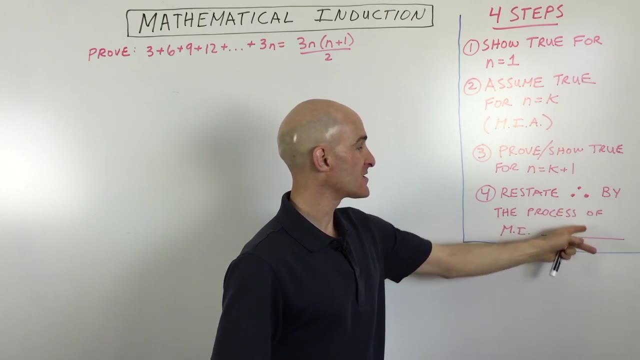 step number three. this is the bulk of the proof. This is usually the biggest part of the proof. The last step is just to restate, therefore, that's what these three dots represent, therefore, by the process of mathematical induction, and restate what it was that you were trying to prove. 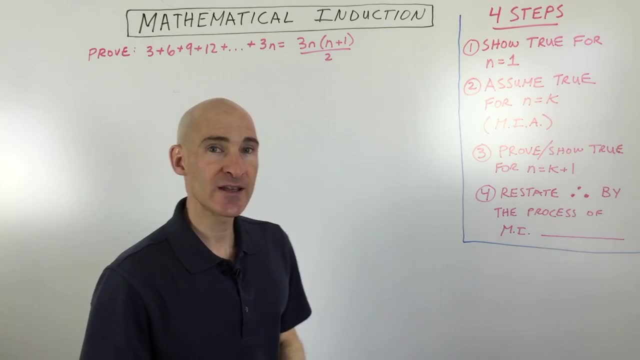 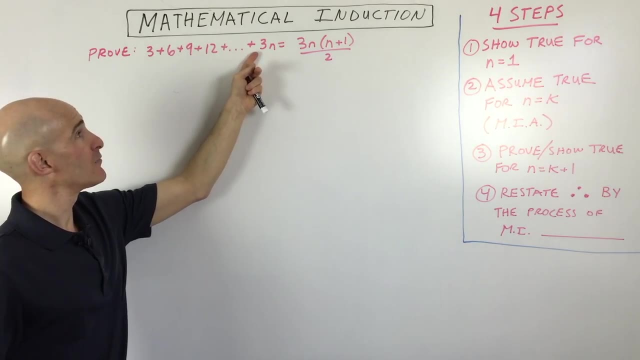 originally okay in the proof. So let's go ahead and get into this example Here. what we're trying to prove is that three plus six plus nine plus twelve plus dot, dot, dot, dot plus three, n okay equals, and this is a formula for the sum of all these terms. 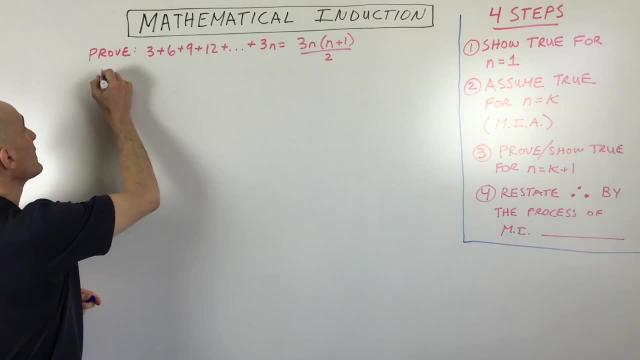 okay. So let's see if we can prove this. So first step, step number one: I'll label this as a formula. So step number two: we're gonna say: let's do two more steps. We're gonna say: show true. 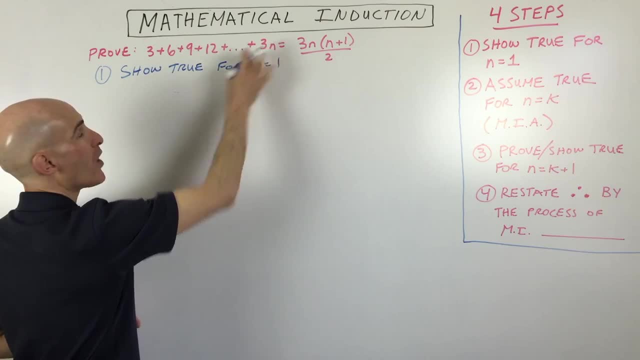 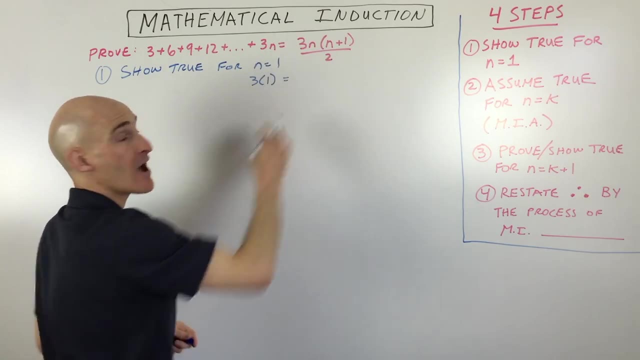 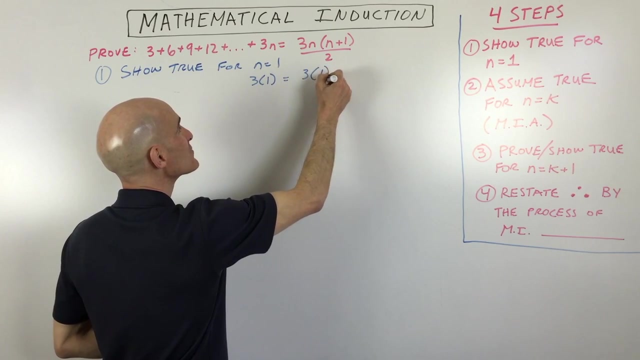 okay, show, true, for n equals one, So I'm gonna put one in right here. This is our formula for finding any term. So I'm just gonna say three times one, and then this represents the sum of all the n terms, In this case just the sum of the first one term. okay, So three times one. 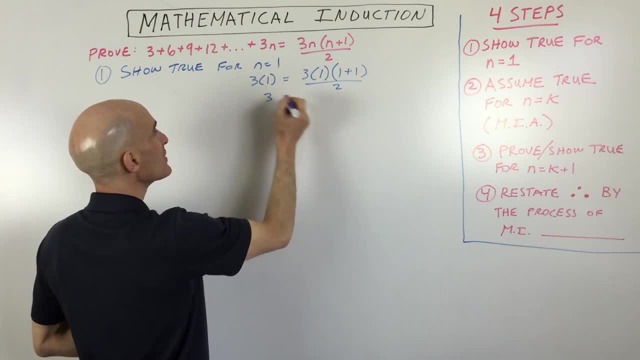 one plus one, all divided by two. So what we get here is we get: and this is three times two divided by two, and you can see the twos cancel. so three equals three. I'm just gonna put a little checkmark, okay, so are you with me? 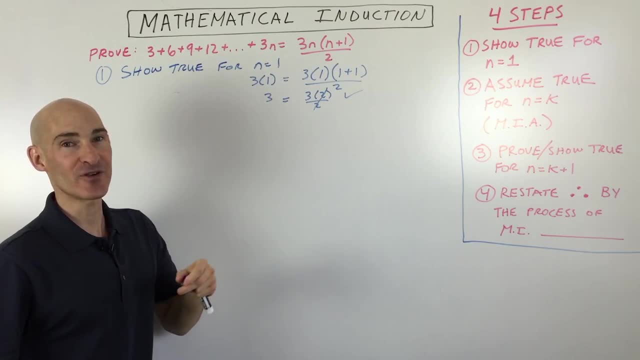 so far. this is the probably the easiest step, right? just to show that it works for the first term. but your teacher could trick you and just give you a formula that just doesn't work and you'd say: well, you know, it doesn't work for the first term, so it's not true, right? okay, let's go to step number two. so step 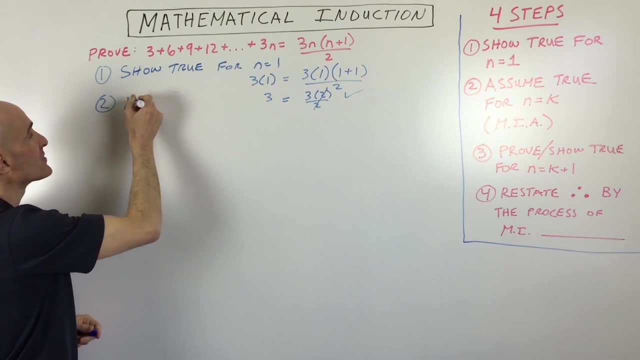 number two. we're just gonna, and you want to, write these little statements in here. this is important for the proof. you don't want to just do it. you want to say, okay, show true for n equals one, assume true. okay, for n equals K. and what I'm? 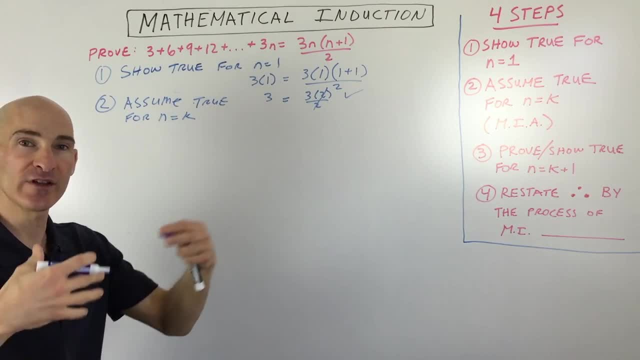 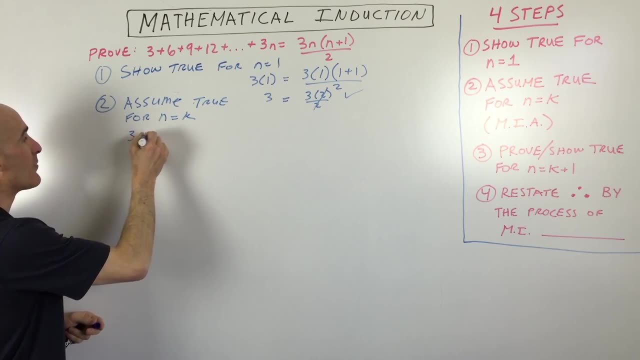 going to do is I'm going to rewrite this formula, but instead of using n, which is more like a generic way of saying n number of terms, you know any number of terms we're going to say more for, like a set number or a fixed number of terms. 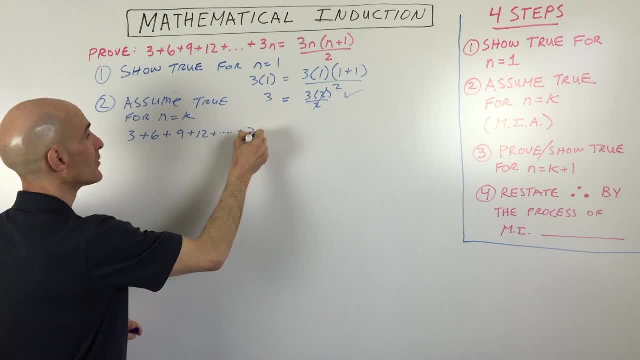 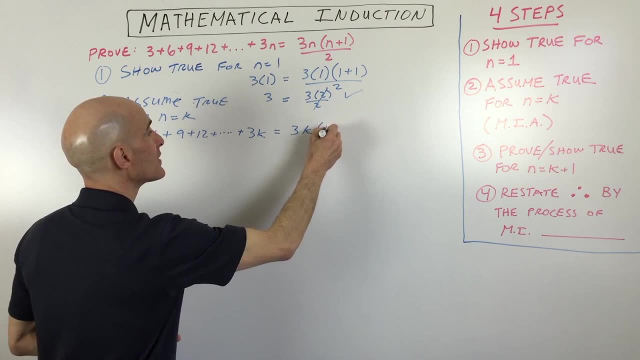 we're going to go up to the k-th term, okay, whatever that represents could be 10 terms, 20 terms, but like a fixed number, okay. so let's go ahead and replace n with K, because we're just going up to two K number of terms. 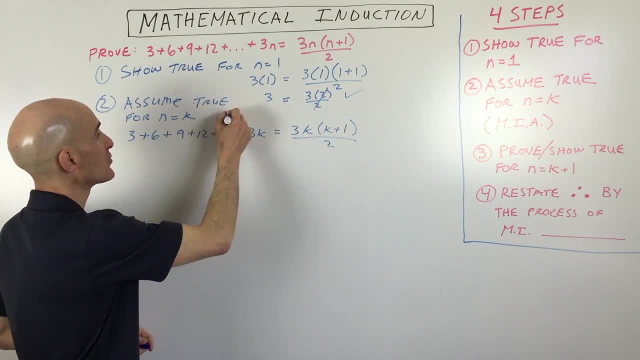 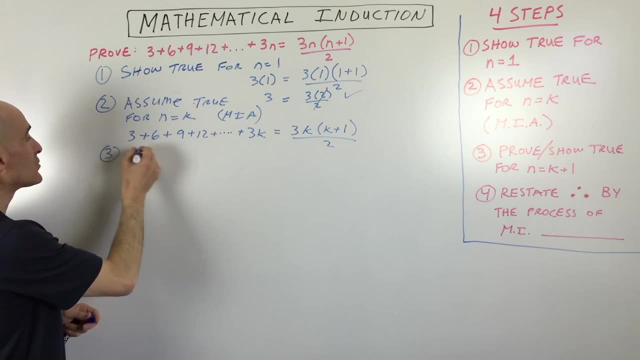 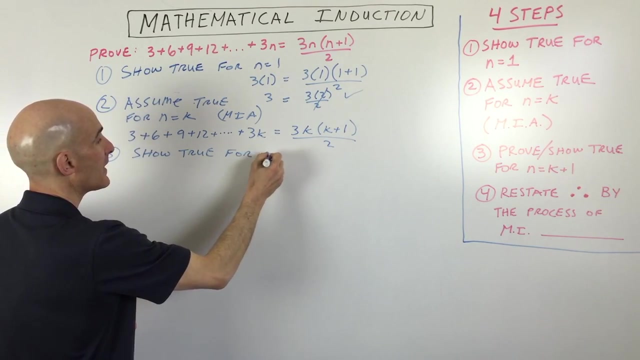 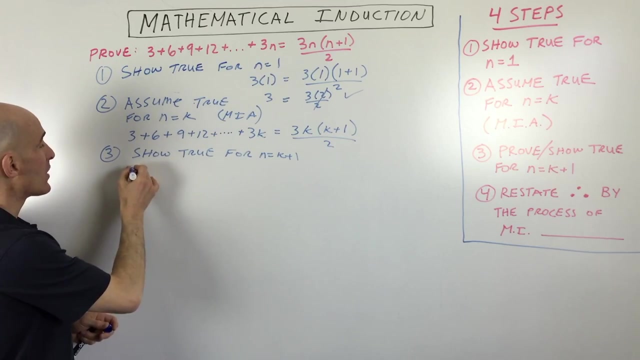 so that's our mathematical induction assumption. we could write MIA here, okay, okay, now we're on to step three. so step three: we're gonna write show true or prove true. okay, for and equal equals k plus 1.. So we're going to the k plus 1th term, the one term beyond k terms. So what I'm? 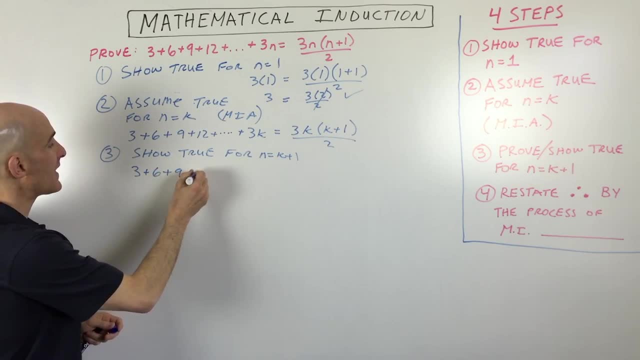 going to do is I'm going to rewrite this formula: 3 plus 6 plus 9 plus 12, plus dot, dot, dot plus 3k. that's up to the kth term. okay, whatever, k is 10.. But now we're going to go one additional term. 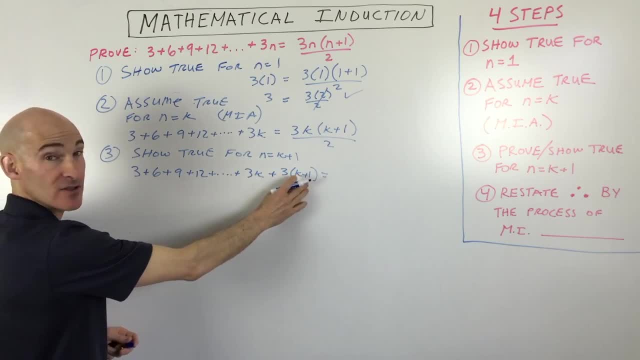 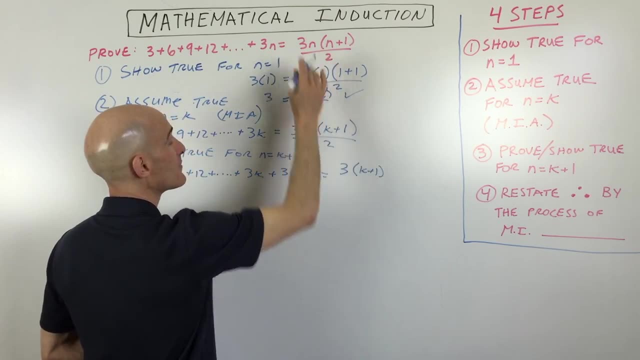 k plus 1.. Now if we add all these terms up to the k plus 1th term, the sum should be 3 times k plus 1, because that's how many terms we have: k plus 1 plus 1, all over 2.. So you can see, I just 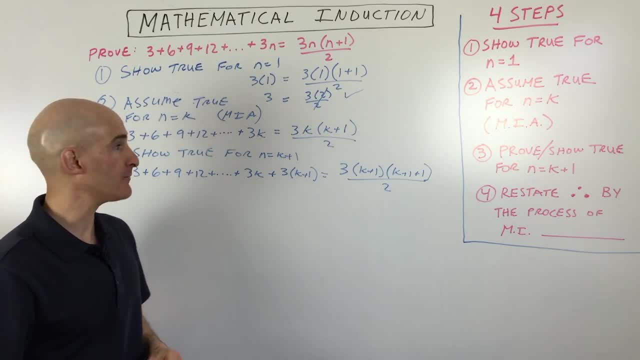 replaced n with k plus 1, because that's how many terms we're adding up Now. this is the bulk of the proof and let me just give you some pointers here. A lot of times students they forget to write this kth term and then to write the k plus 1th term. They'll just go right up to k plus 1,. 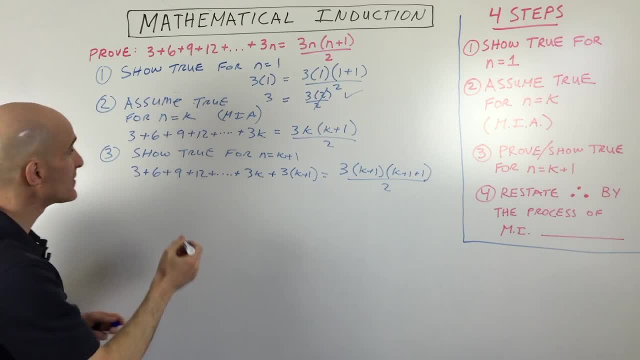 skipping over this term. So you want to write all this, and I'll show you why The reason is is because you're going to have to write all this, and I'll show you why The reason is is because you're going to have to write all this, and I'll show you why The reason is is because 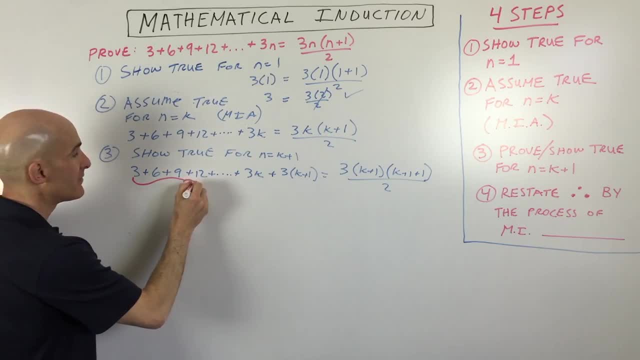 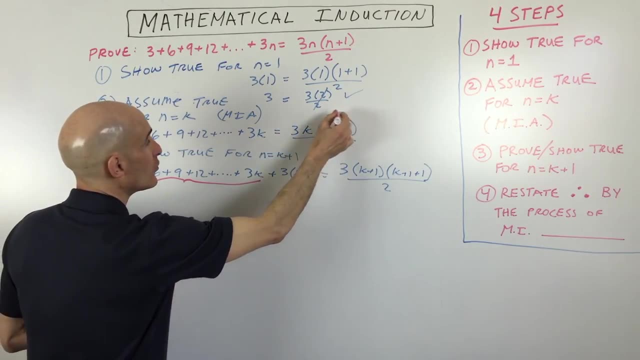 what we're going to do now is we're going to say: all right, the sum of the first k terms, right here. what does that equal? Well, we can see here from the previous step: it equals 3k times k plus. 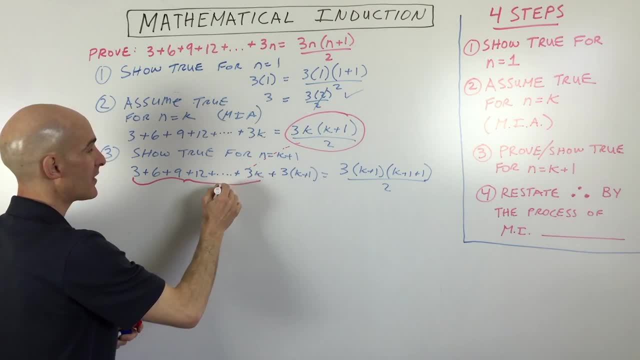 1 divided by 2.. So what we're going to do is we're going to replace that. okay, right there. The sum of these first k terms equals this. So we're going to write that right here: 3k times k plus 1. 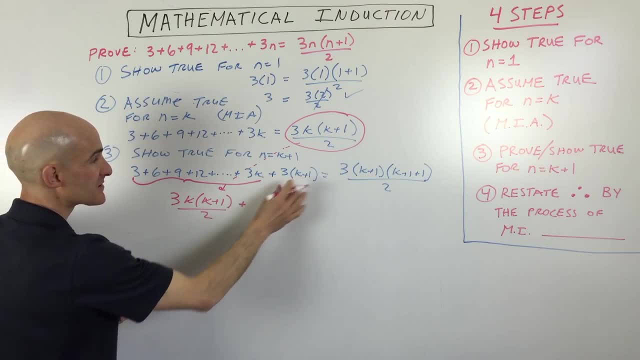 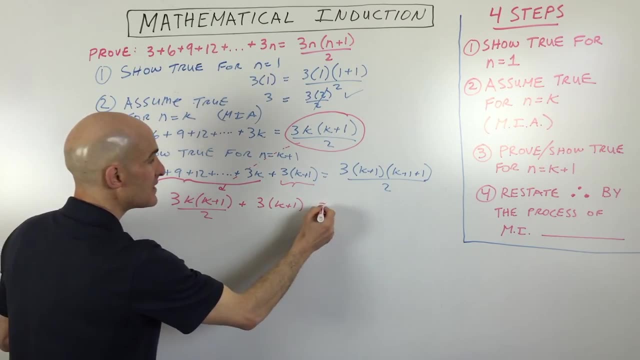 divided by 2, okay, plus this term here, that's our k plus one term. three times k plus one equals, and we're trying to show that it equals this right here. okay, so you're with me so far. so this is just algebra and I. 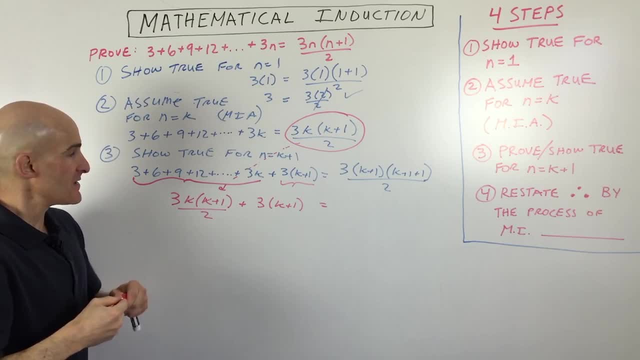 just want to state something here for you that you don't want to necessarily foil and multiply all this out. what you can do sometimes is you can take what you have right here and work with that. you can say: well, hmm, I know that I'm trying to show that it equals this. I can see I already have. 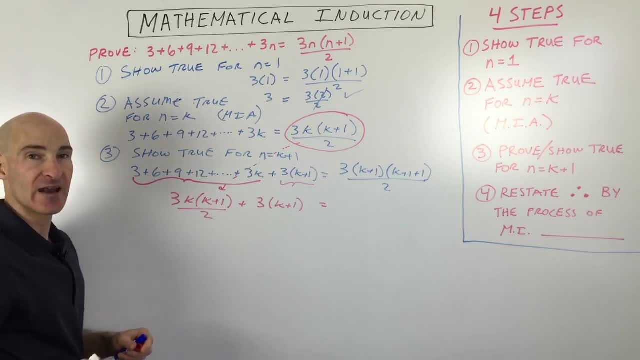 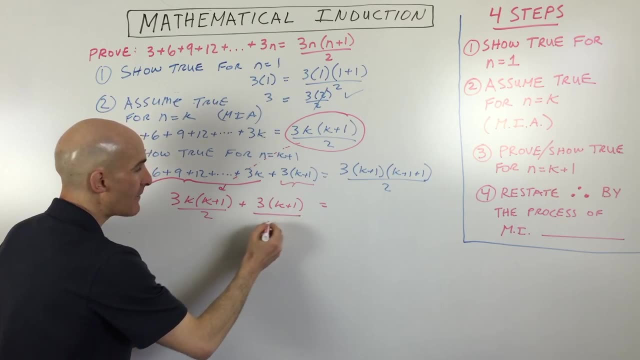 a k plus one in both of these groups. maybe I can factor that out so I don't have to multiply this out and then try to, like you know, factor it from there. but what I'm going to do here is I'm going to multiply the top and the bottom times two. okay, this way we get a common denominator. okay, so now? 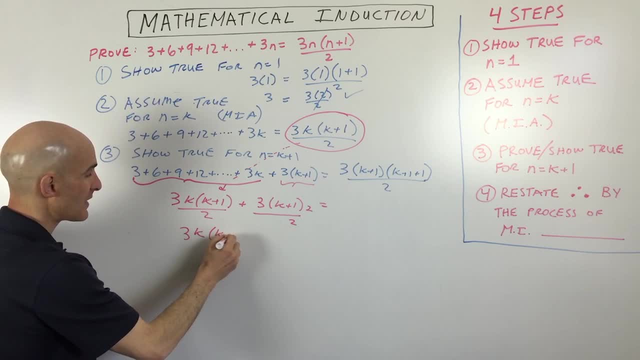 if I can just rewrite this, we've got 3k times k plus one plus six. okay, because two times three times k plus one, all divided by two, we got a common denominator. okay, now when you look at this group and this group, see how you have like a three in common. you can. 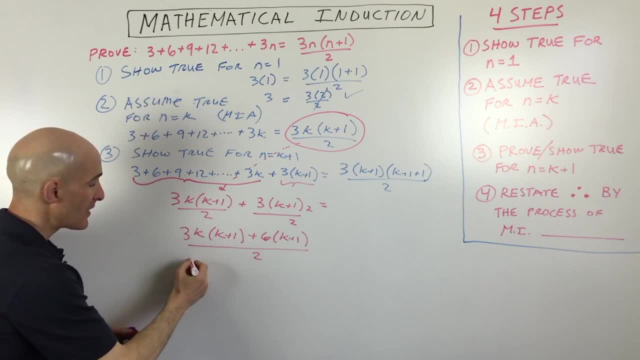 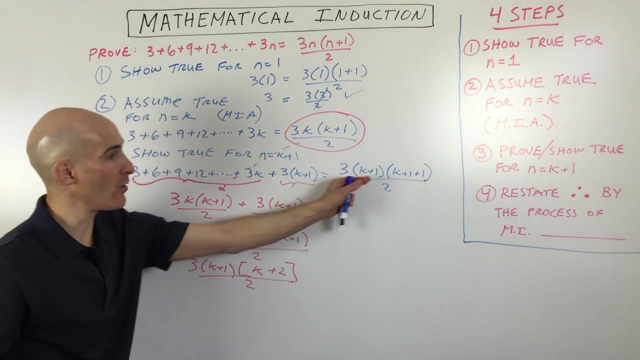 factor out and a k plus one. let's factor that out. so what we have here is we have three times k plus one times we're left with k from this group plus two from this group, all divided by two. now you can see we're almost there. all I'm going to do now is I'm just going to rewrite k plus two. two is the. 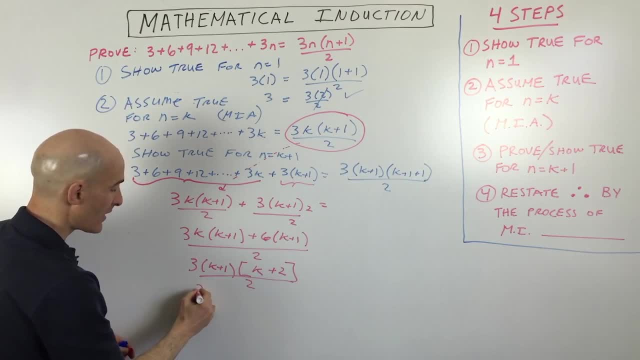 same as one plus one. so I'm just going to rewrite that and I'm going to do that again and I'm going to just going to break this down so it looks a little bit more like the right side. so we've got k plus one times k plus one plus one, all divided by two. okay, so now we've proved it. you can see that these are. 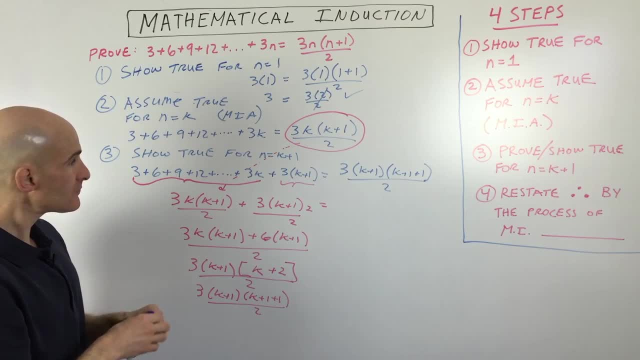 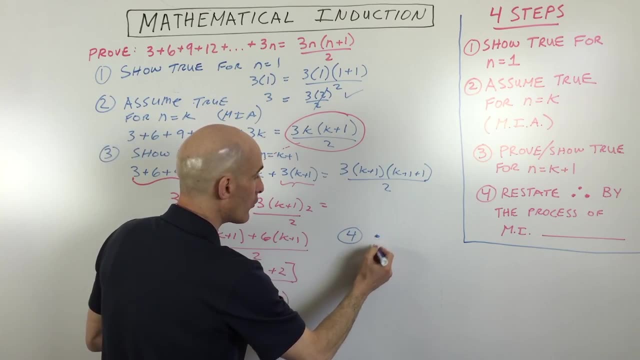 the same. so the last step, step number four, is to restate what it is that you were trying to prove, so I'm just going to put it right here. step number four: therefore, okay, there's a lot of different symbols that you can use, but this is a common one, so I'm just going to put it right here. step number: 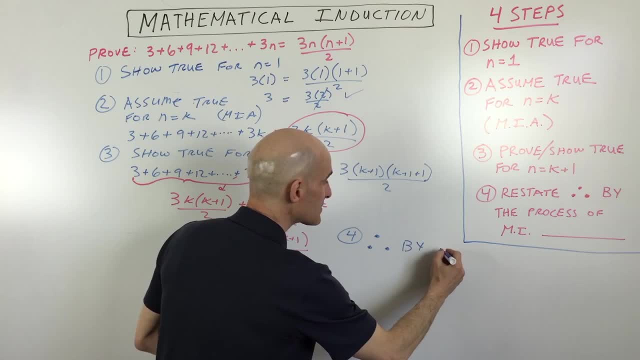 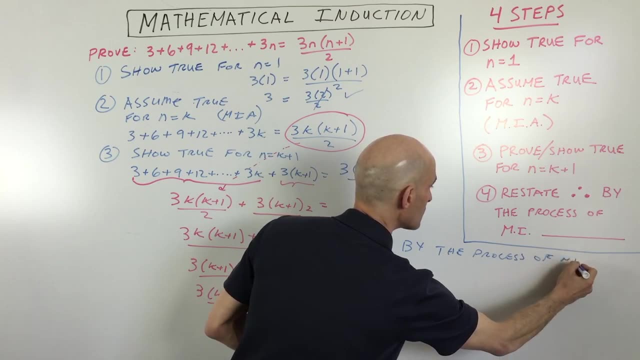 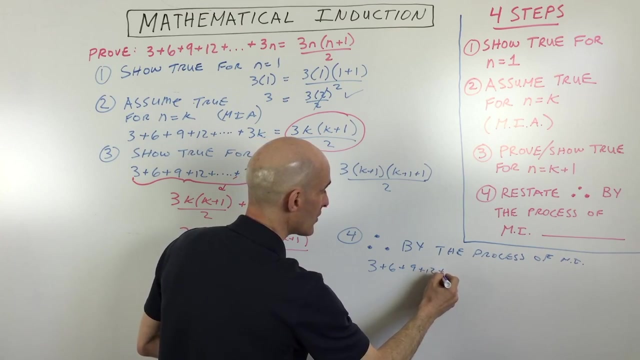 one. therefore, you can say by the process- okay, by the process- of mathematical induction, and then what I'm going to do is I'm going to restate what it is that we were trying to prove: three plus six plus nine plus twelve, plus dot, dot, dot plus three, n equals. 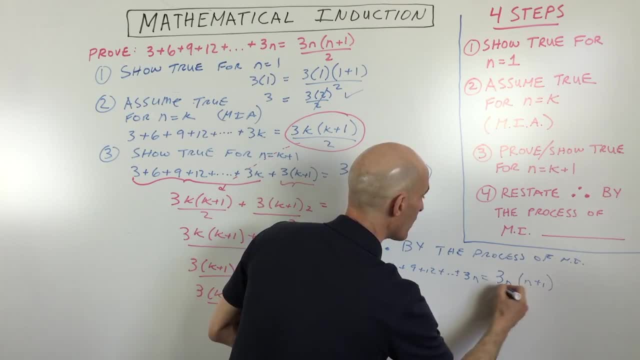 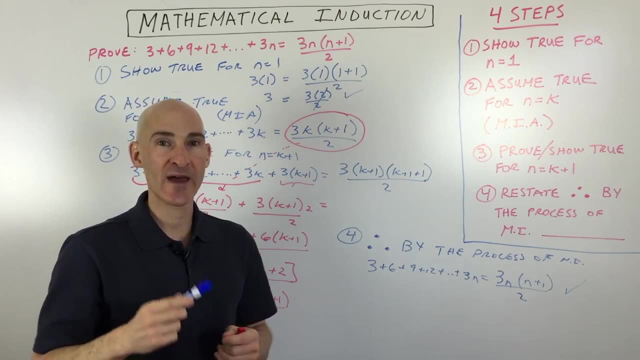 and the formula for the sum is three n times n plus one, all divided by two. and that's it we proved. so let's take a look at another example. I'm going to erase the board and I'll be back in half a second, okay, okay, in this next example, what we're going to do is we're going to prove this other theorem. 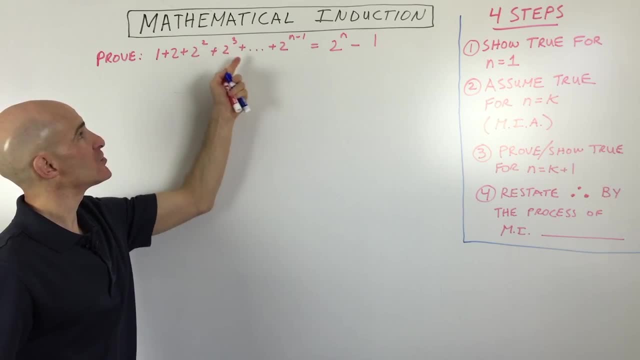 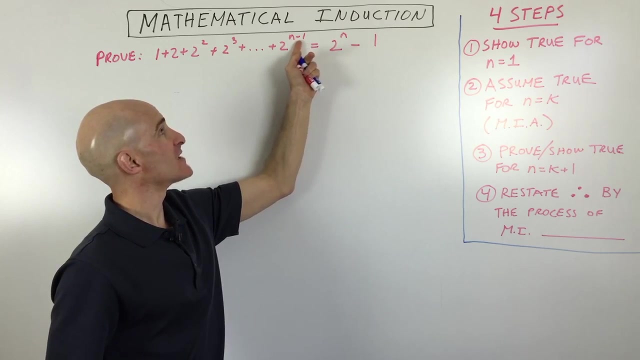 here, which is one plus two plus two, squared plus two, cubed plus two to the fourth, plus dot, dot, dot, all the way to two to the n minus one power. if you were to add up all these terms, we're going to show that the sum equals two to the nth power minus one. so notice this: n minus one is an exponent. 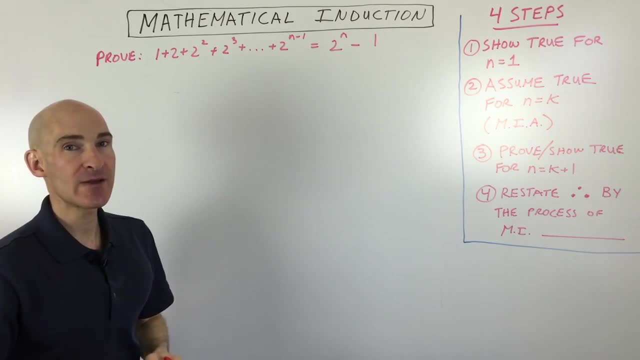 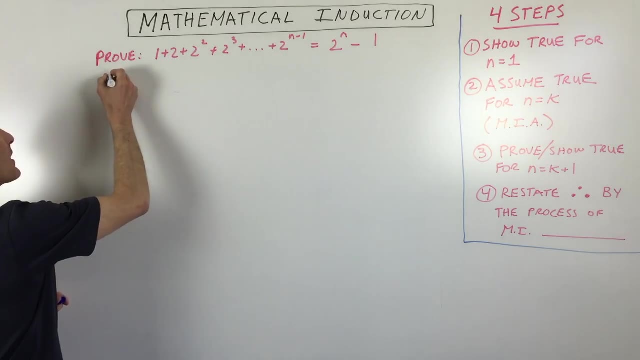 this minus one is just over here to the side. so we're going to go through the same four steps. step number one: we're going to show that it's true for n equals one. so let's do that here and I would write again these steps out. I would say step number one. 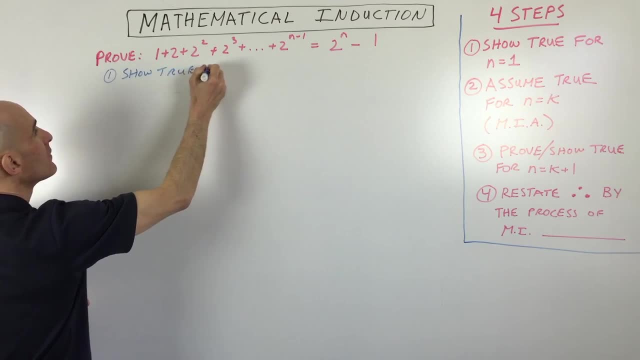 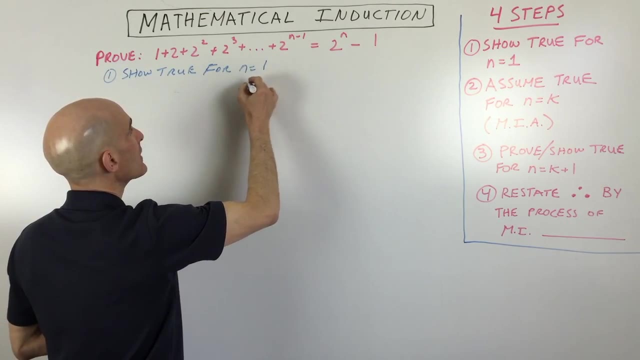 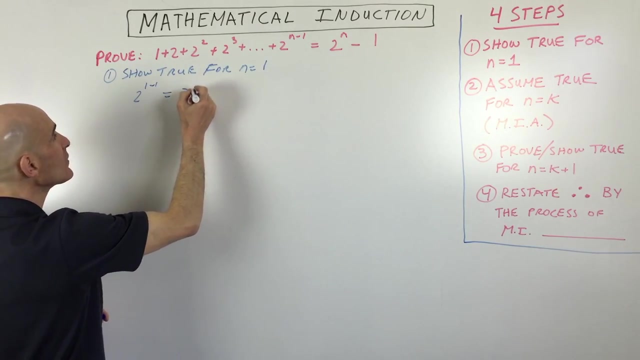 show true for. okay, for n equals one. so I'm just going to put one in for n here and I've got two to the one minus one equals, and this is the sum of the first one terms, which is two to the first minus one. one minus one is, of course, zero. two to the first is two, anything to zero power is one, and two minus one is one. 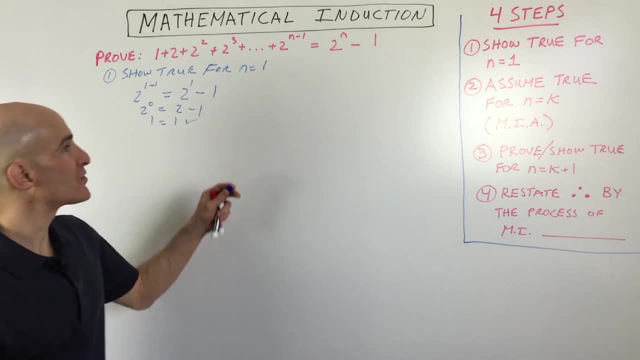 okay. so step number one done. okay, so now step number two. we're going to assume true for n equals k. this is our mathematical induction assumption, and we want to start off by writing that we're doing that. so I'm just going to abbreviate mathematical induction assumption one plus two. 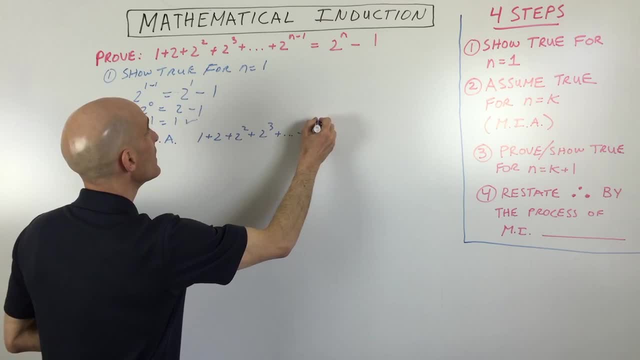 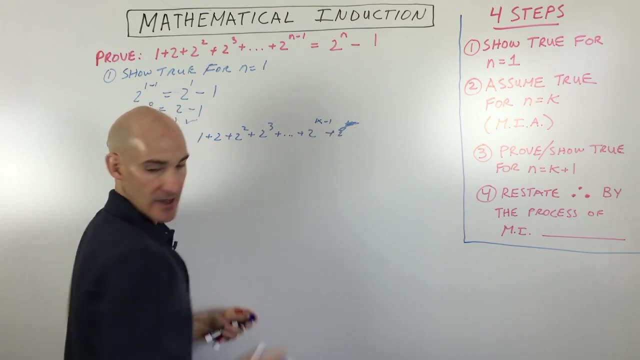 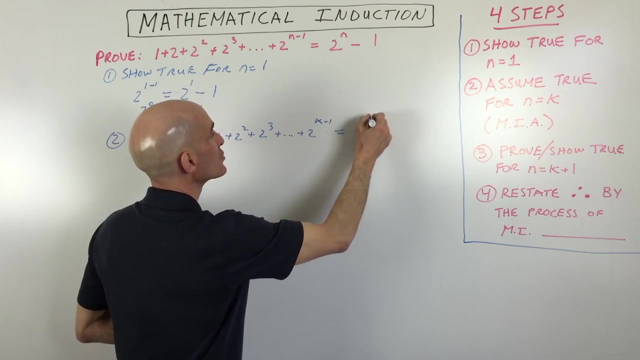 plus dot, dot, dot, plus two to the k, minus one plus two to the k. well, let's just go right to there. okay, stop there for a second. so we're all we're doing is replacing n with k, so we're just showing that it works for the first k terms. okay, so all we do is replace n with k and we're just saying that the 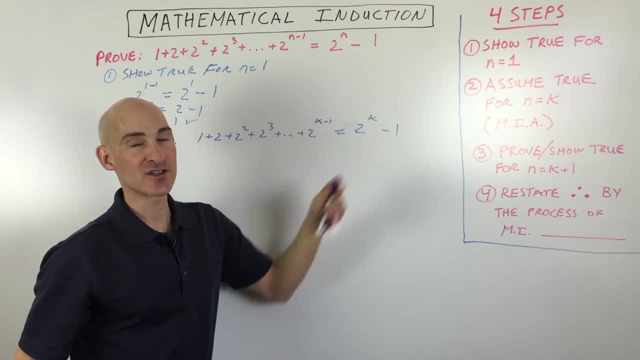 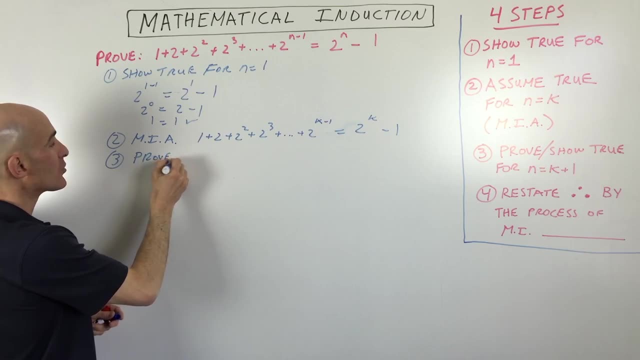 sum of the first k terms. this is true, so that's our assumption. so that's done. now step number two, three. here's where the bulk of our proof. we're going to prove true or show true. okay, for n equals k plus one. okay, so now we're going to go beyond the kth term. one additional term, if it works for. 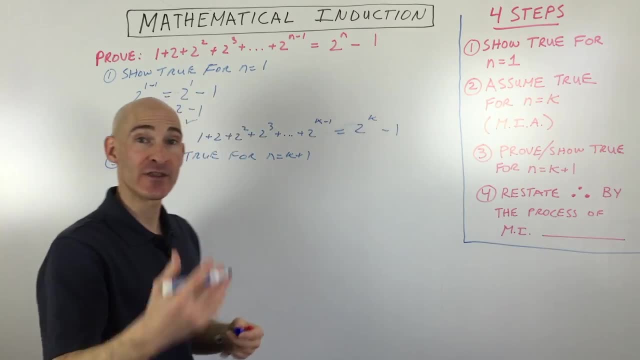 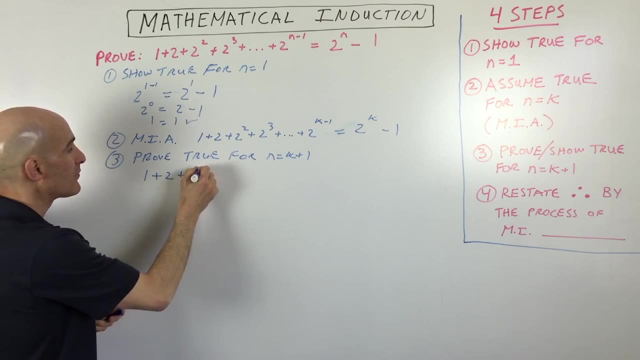 that it's going to work for one beyond that, one beyond that forever and ever. and then we've proved it so by the process of mathematical induction. so let's do that. we've got one plus two plus two squared plus two cubed, plus dot dot dot. 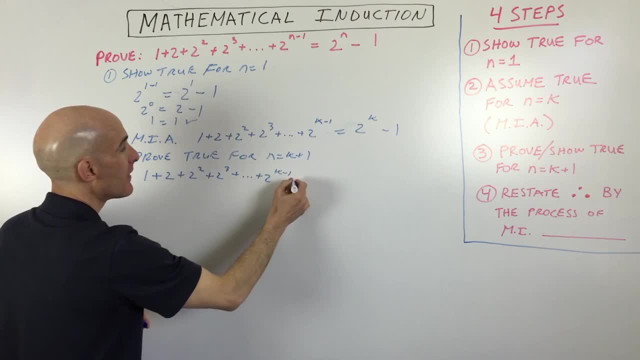 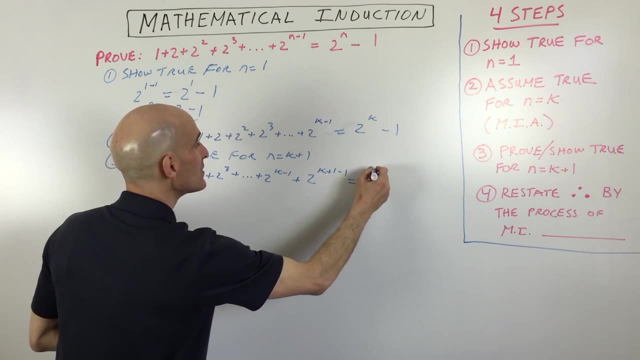 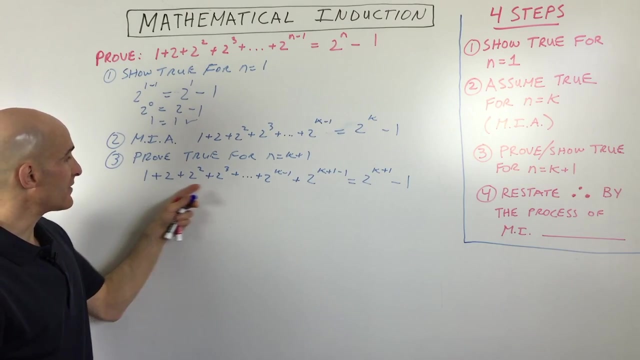 plus two to the k minus one. that's the kth term plus. we're going to go one more term beyond that. two to the k plus one minus one equals two to the k plus one minus one. okay, so just to restate, this is the first k terms. this is the k plus one term. I put k plus one in for n because n is.